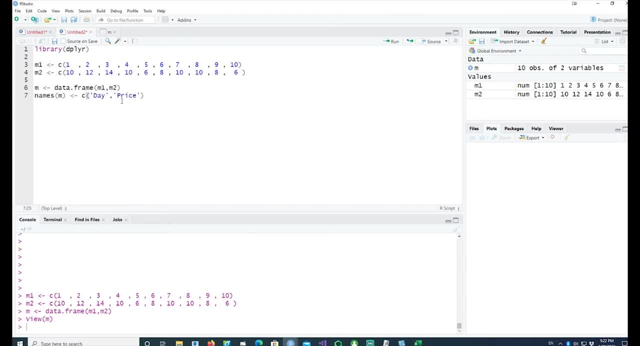 Okay, so I'll call them as day and price, If I can go back to m again. you can see we have 10 days and the price of a fictitious share. So let's try to work on this and see how we can. 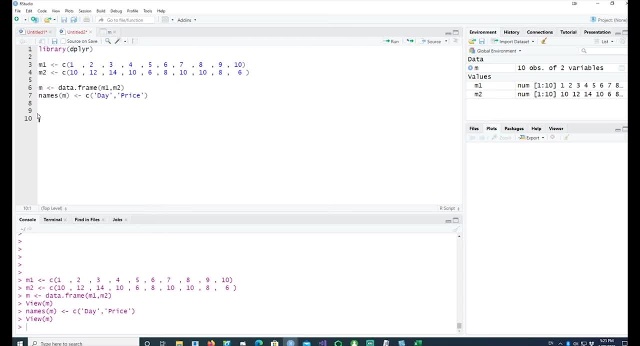 do a few things in terms of calculating the rate of change or the change. So, using the dplyr, I want to construct another data frame called mc and I'm using this pipe command. There's a concept in dplyr which we can use, which is called: 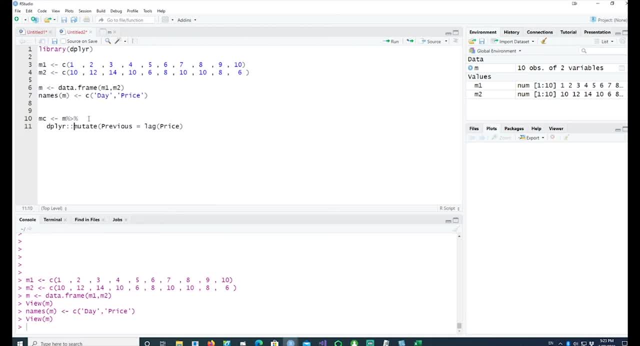 dplyr. So there's a concept in dplyr which is called the lag. So lag simply means the value of a variable in the previous row and it's called lag. And let me run it so that you can appreciate how it works. 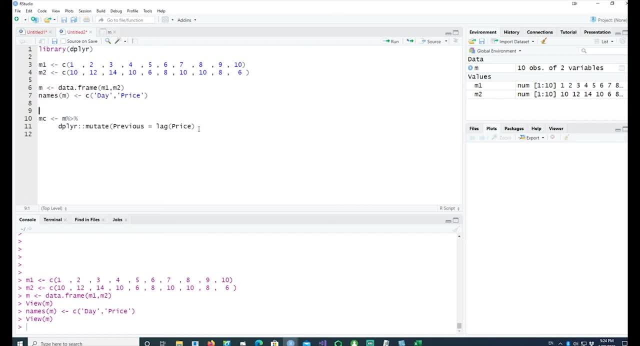 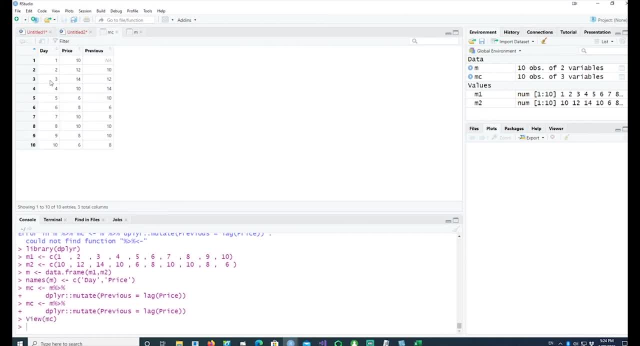 We've got a third column in our data set, So we have the price And we can see we have a new field called a new column, called previous. So previous has actually put the data from the previous data into this column. So if I look at the sixth row you can see that this value has come from there. 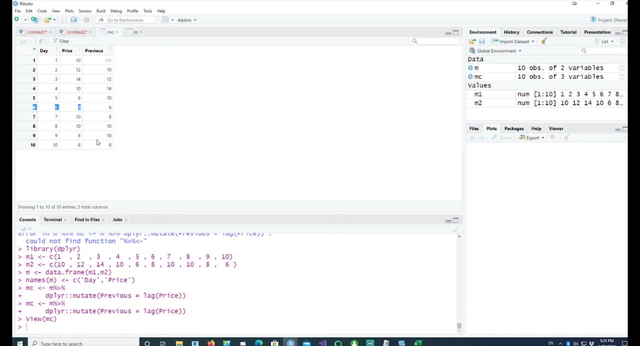 And this value has come from there And this value has come from there there. so the the the previous period data has been put using the lag and similar similar to lag. you can also use the next. if I wanted the price of the next day, I can call it as lead. 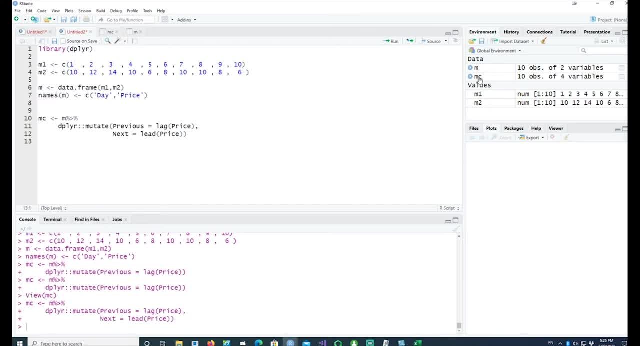 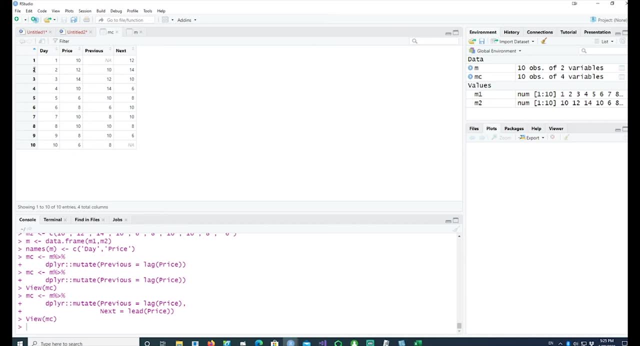 and see what happens. so we got MC and here we go. we have a previous period data and then the next one's data as well. so in the in the road to, we have got the data from row one and also the data from row three. now we can simply 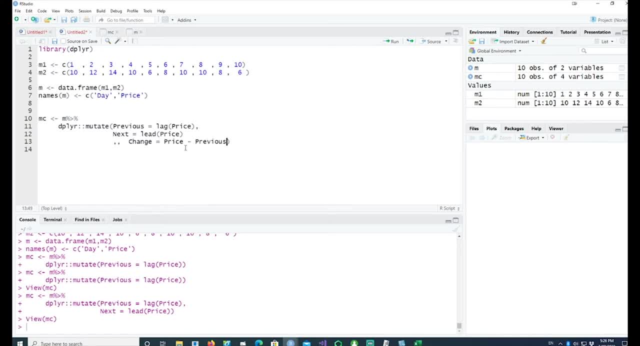 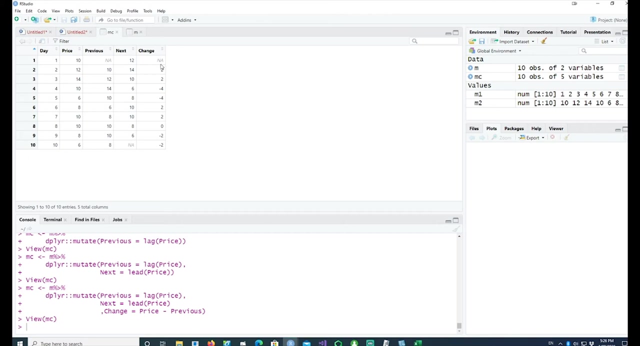 calculate the change by doing this subtraction from today's price from the previous day's price. so here is a change. obviously on day zero or day one there was no change. on day two we start subtracting today's price with the previous period price two. so in this case, for example, this 10 minus 14 gives 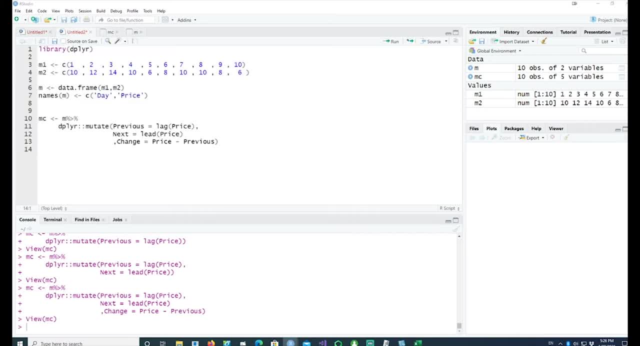 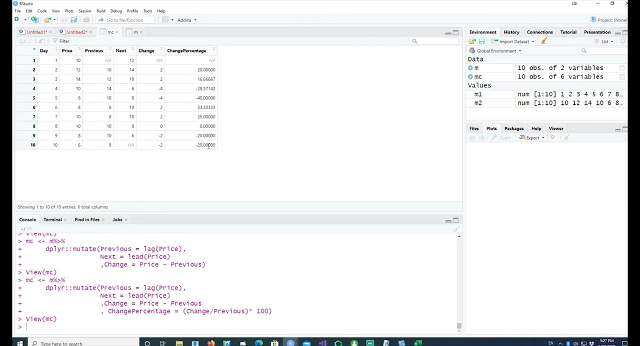 us negative four, and if I wanted to convert this change into a change percentage, I could simply multiply it by hundred and I'll get that in the column. so here we go. that rate has been converted into a percentage. now we could have simplified this instead of calculating the previous and then. 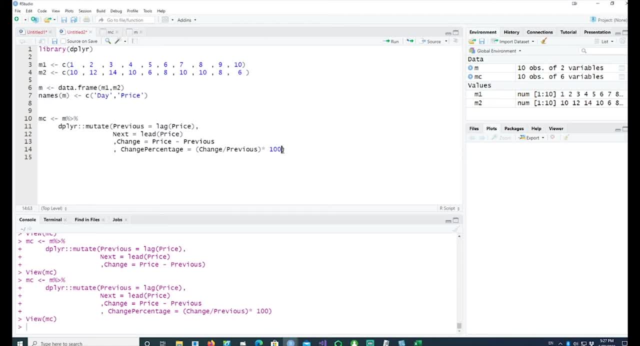 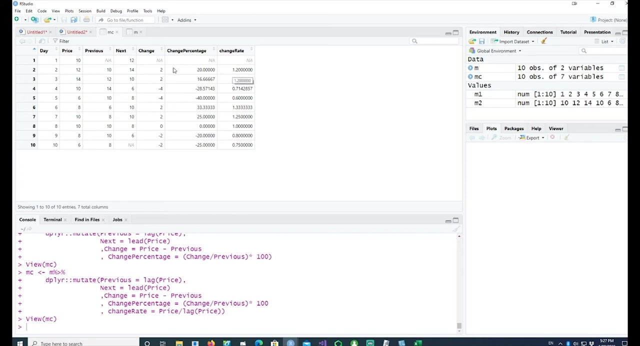 calculating the next, and we could have simply done the whole thing in one simple statement, and that would have been just saying price divided by the price, and that will give us a rate as well. so this is the change in terms of. so if you multiply 10 with 1.2, you're going to get 12. 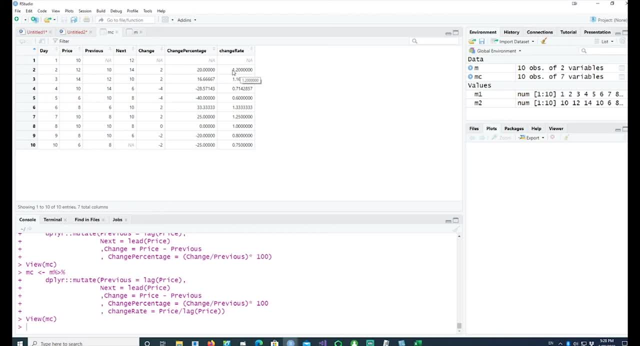 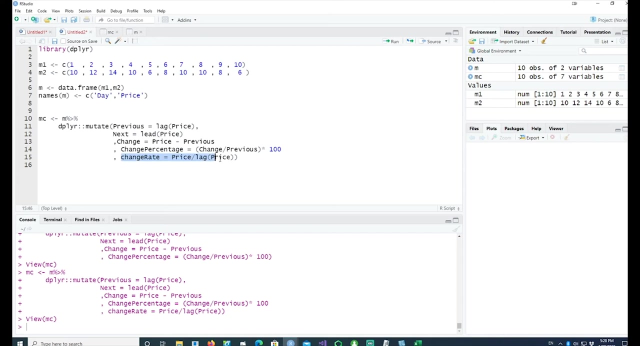 so if you multiply 10 with 1.2, you're going to get 12, and if I wanted to get the percentage change, I could have done price divided by lag price minus 1 and 200, so it gives us the same thing instead of. 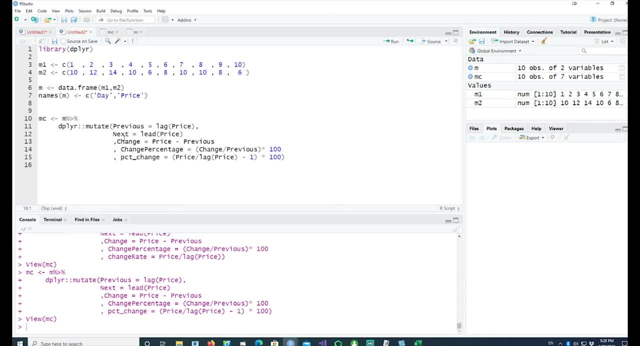 calculating it separately by calling the previous and then next. I can simply say price divided by lag price minus 1 and multiplied by 100. And if I wanted to see how my share is performing the day one when I bought my share, I can do that as well. for example, I can create a field called day one: everything gets offered. what I'm getting at between the last two terms of the day is the first thing: each rate cook forwardena price bulleted into 1.2 and each timestory price shopping in the next page you're going to hit the flowers and price valueなもの give and multiply by no zero. And if I wanted to see how my share is performing the day one when I bought my share, I can do that as well. for example, I can create a field called day 1 price and that will be the first rows to awareness. buy interest rate set to occur. 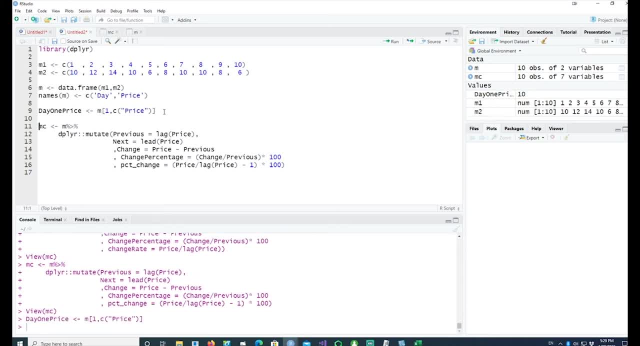 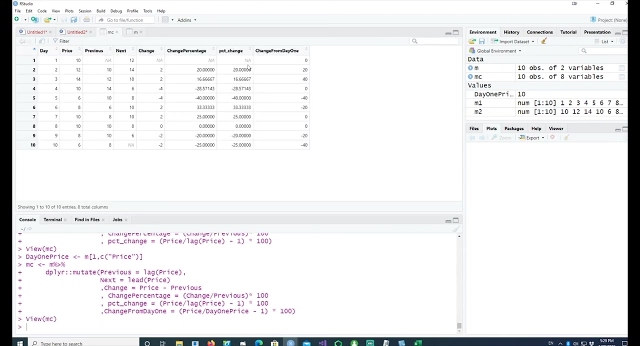 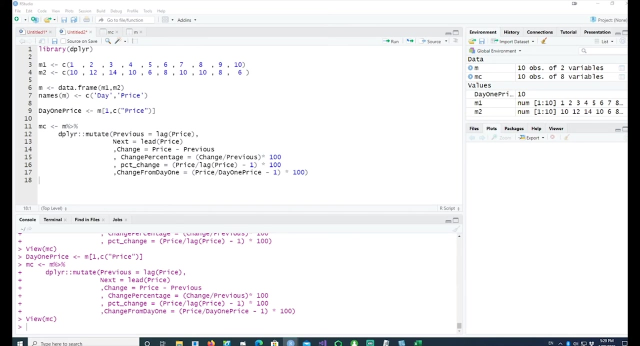 hopefully we should have this. yeah, so day one price is 10. that's good. we can use that and calculate. so if i look at mc, i can see that this has been my change overall. on the day 10th, my share price is down by minus 40 percent, which from 10 it has gone down to 6.. how about plotting this? 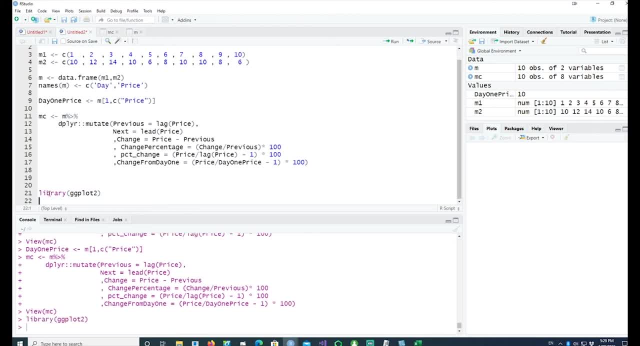 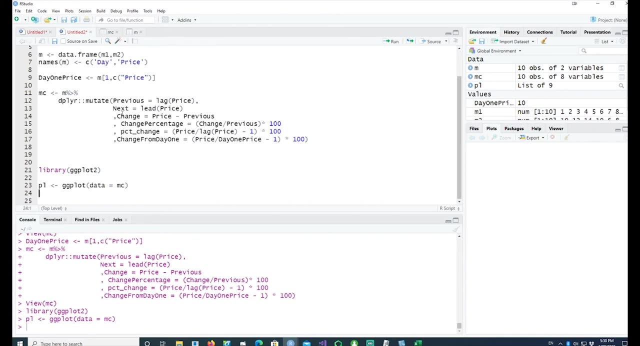 change. so let me use the ggplot package and i'll use ggplot. data equals mc, the data data frame which we have created, and we have calculated our changes in a different, in different fashion, and i would like to use a line plot, calling the geom line and using x. 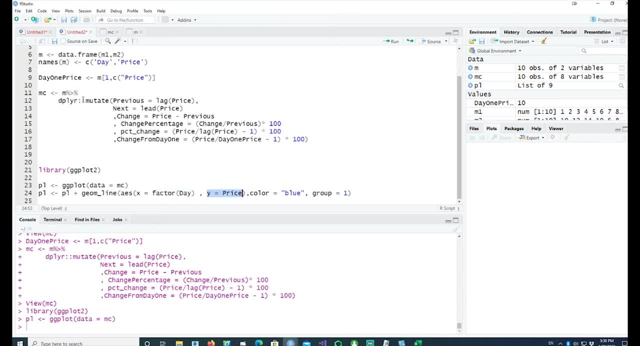 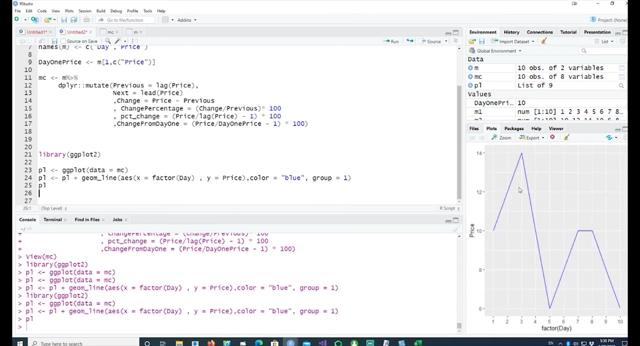 as the factor of the day and y being the price of the share, and i want to give it a blue color and group equals one, and if i run my chart i get a line chart. let me use a theme to make it a bit more clear. so here we go. we have a theme, classic, okay. so this is our simple line chart. 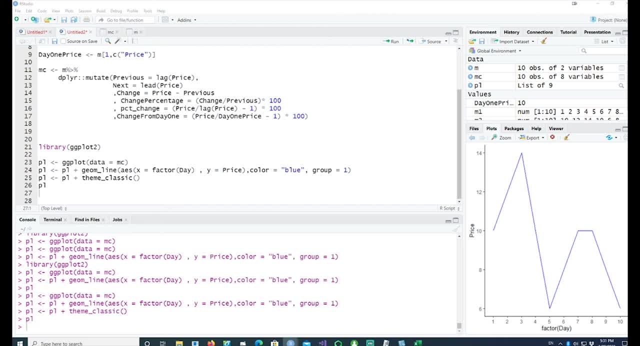 what if i wanted to plot some dots as well? all i had to do is give a jump point so that i can get a line chart, and i want to plot some dots as well. so i'm going to create a statement with x and the y aesthetics for that. 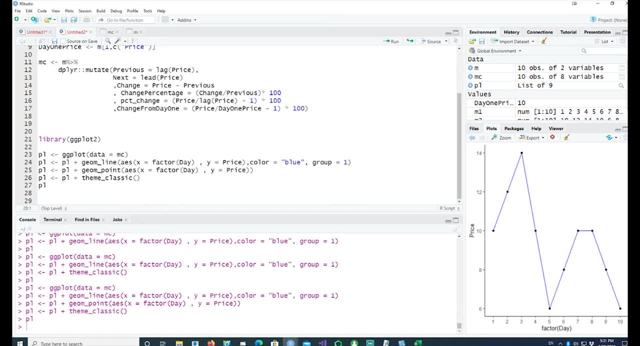 okay, here we got the, the line going and the dots or the points coming as well. now let me bring in the percentage change in this as well. so, if i can put it up here, i want to have a geom call or the column. again the same thing: x equals the day, but in the y i want to have the. 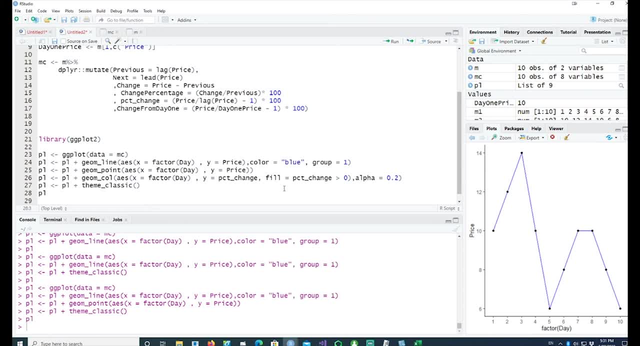 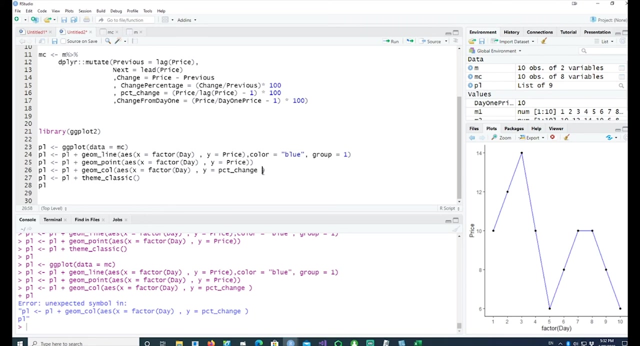 percentage change or the pct underscore change, and i want to fill the percentage. let me remove this for the time being. let me make it simple and run it for you. okay, let's have this percentage change plotted as a jump call as well. so if i run this whole, 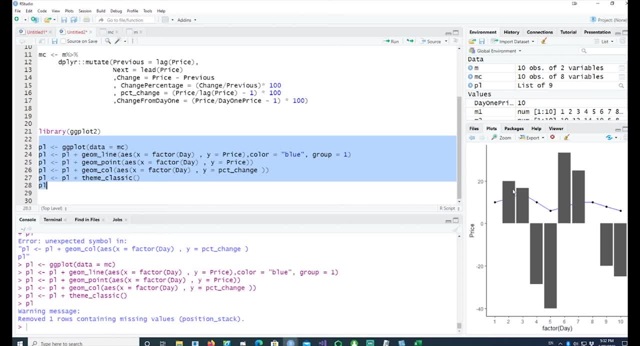 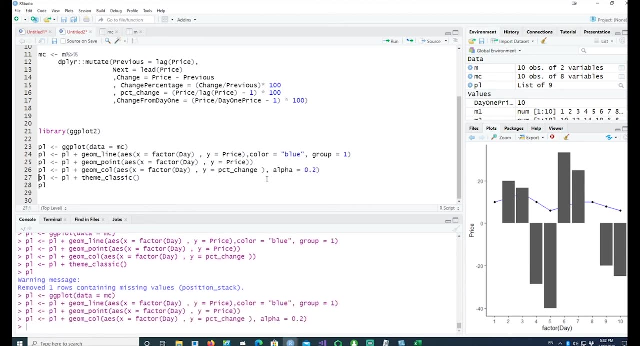 statement, you would see that a bar plot has been created on the line chart as well. we will have to reduce the transparency to make a bit more sense into that, and i can put an alpha statement there. to make our bars a bit more transparent, we can also change the color by giving a. 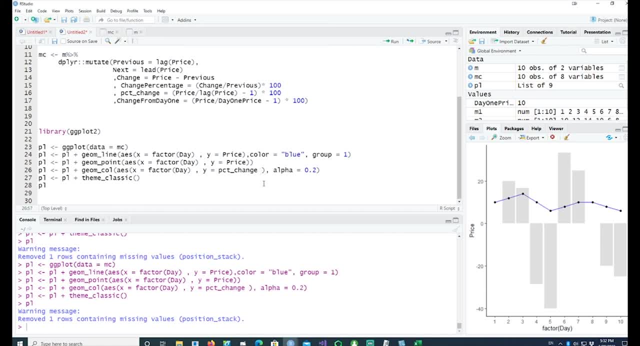 a fill option and i can say fill and i can give a conditional fill saying percentage change equals or more than zero. if the change happens to be more than zero, then we would color it differently compared to when it's negative. so let's run and see the results. so it has given us two colors. 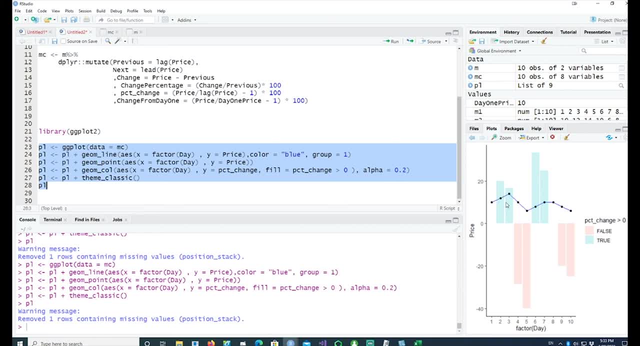 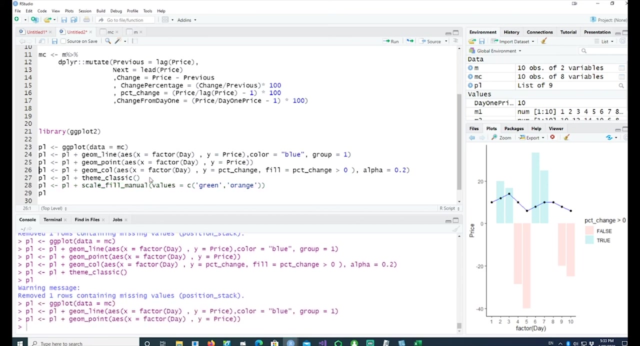 blue or green, blue or red or green or red. i can bit, i can make some, some more changes to that. what if i wanted to have the color controlled as well? i can give a scale fin manual and see what happens. now you can see that scale fill manual has given us. 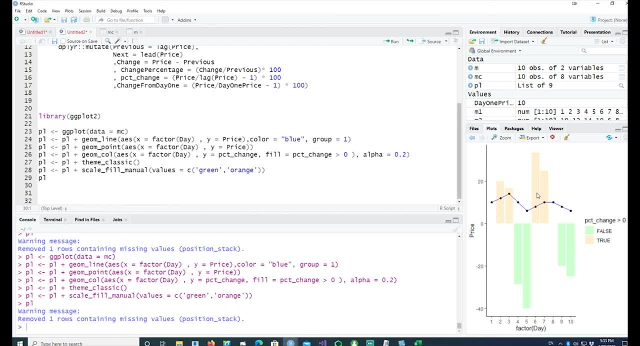 green and orange instead of the previous colors which you were getting. we can control our true color or, when this condition is met and when this condition is not bad, by giving two sets of colors in there. i can also just select the color in our class and it will give me two colors. 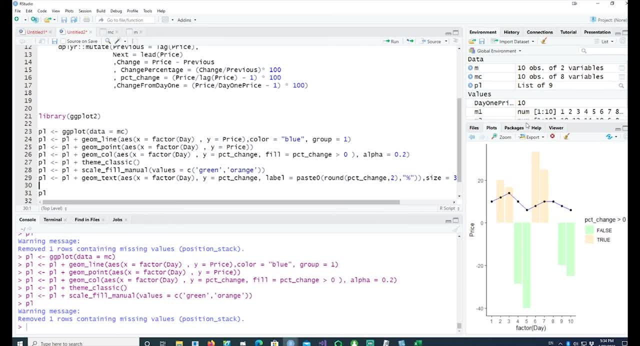 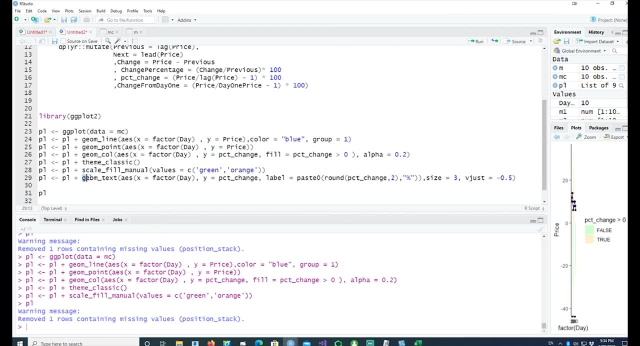 so if i wanted to see what my percentage change has been now? what if i wanted to see what my percentage change has been? to make it simple, we are simply saying i want to have some text, and this is the location for the text: x equals factor day and y equals percentage. and what do we want to print it? 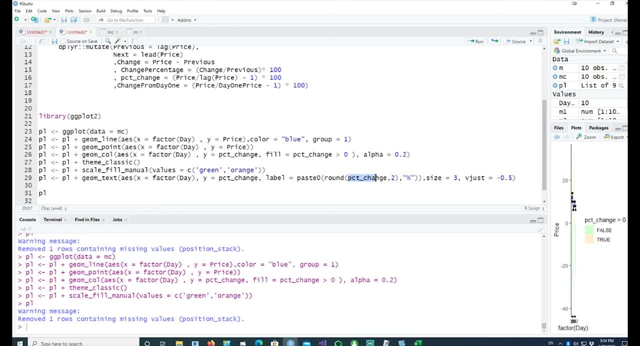 we want to print the percentage change and i want to round it by two digits and i want to place a symbol of percentage after that, so that pay statement is going to give us that and the size. i just want to make it size 3 and i want to be justified by minus 0.5. that puts the 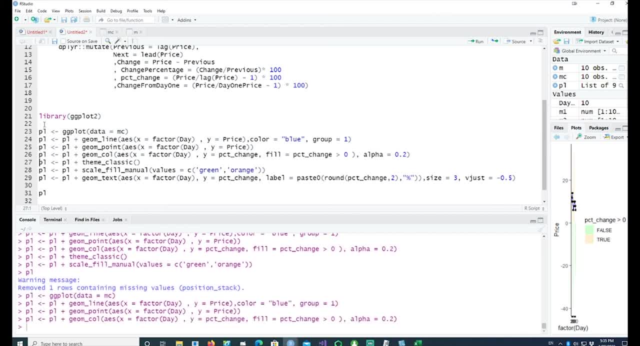 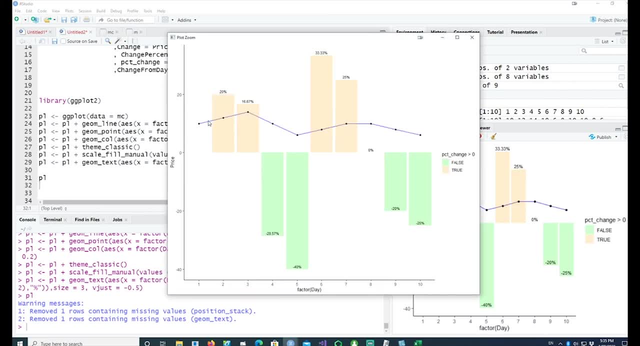 the text bit higher than where the the bars finish. so if i zoom it for you, you can see that the text has been placed at the right spot. again, we can adjust these points by using different uh v justifications. we've used minus justification there. we might have. 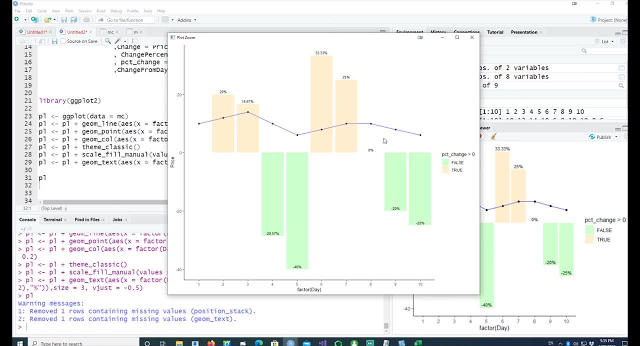 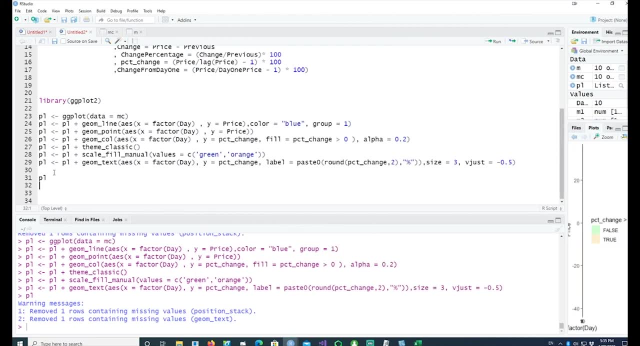 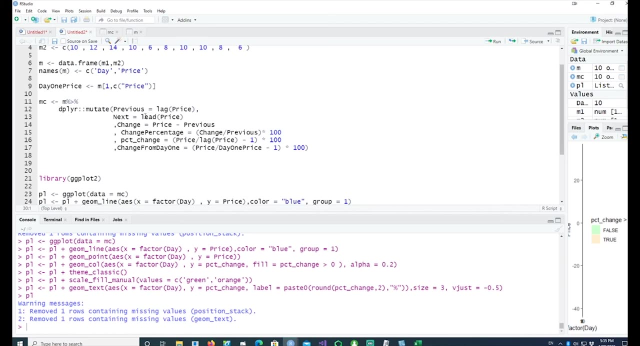 to increase it to to plus justification, in this case to bring it down. you can play with that. so this is um. this video has given you some idea of how you can calculate the, the previous period or the next period information in your current record. you can use that to. 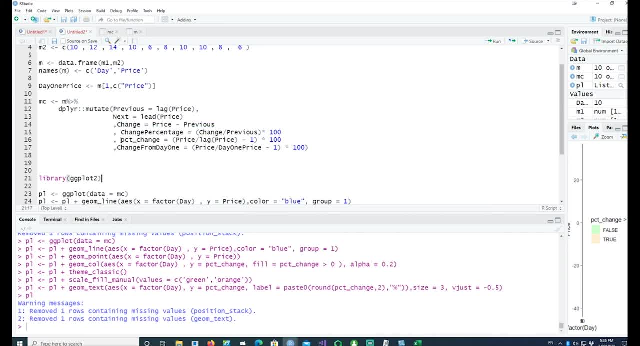 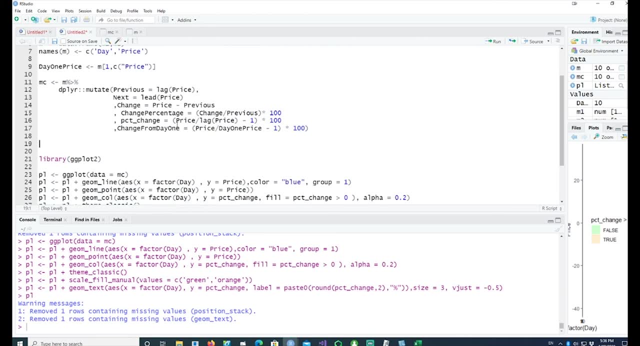 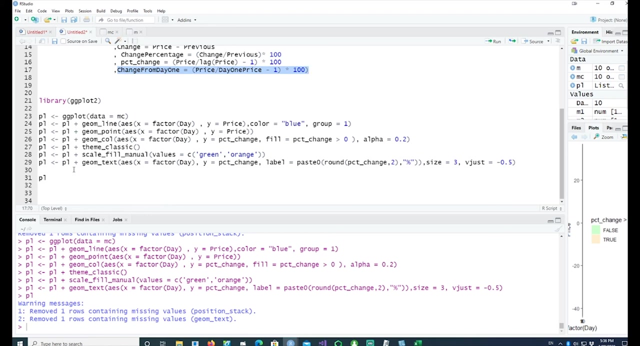 calculate your change. you can calculate the change, uh, by change, converting it into a percentage, and there are different ways of doing that. and then we saw how we can actually do a change from our given point, for example, in this case, the the first day's price. and with that we come to the end of this video. hope you got some useful information out of this.